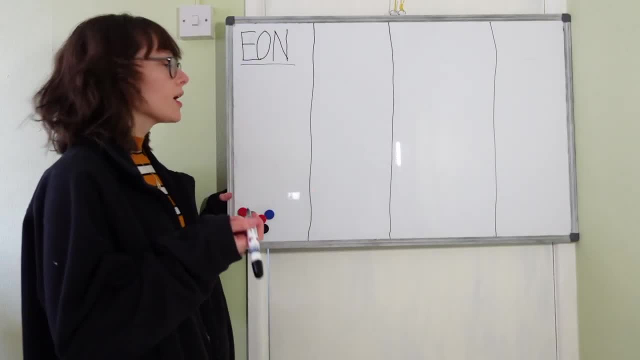 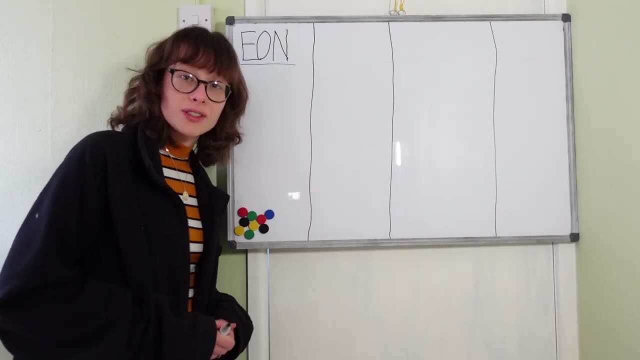 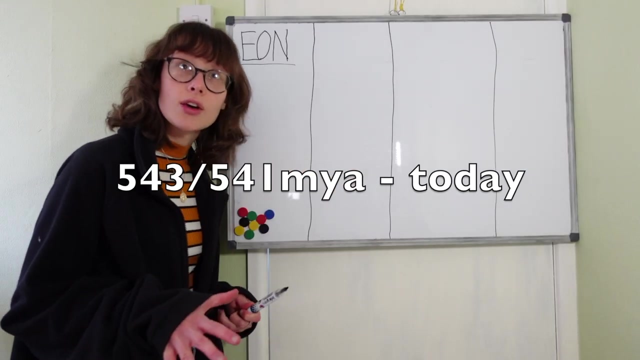 However, just to keep it simple, we have the pre-cambrian, which spans for 88% of the Earth's current history, and the phanerozoic, which spans from 543 or 541, depending on who you ask, million years ago to the current day. Now, for exemplary purposes, I'm just going 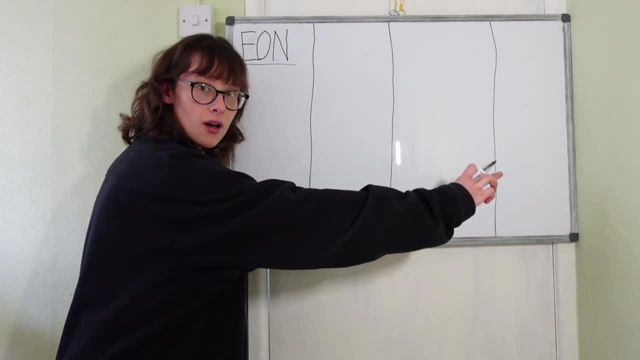 to write the phanerozoic here so we can divide that up as we go along. Right, next, we are moving on to an era. 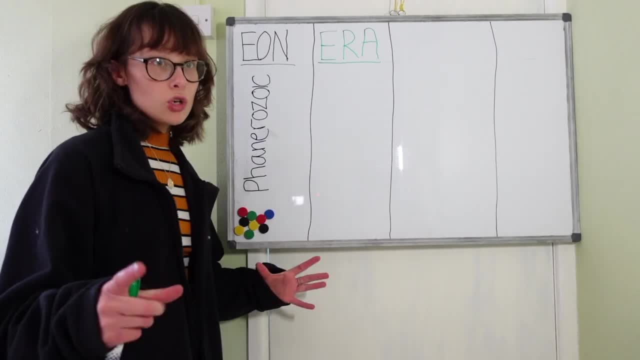 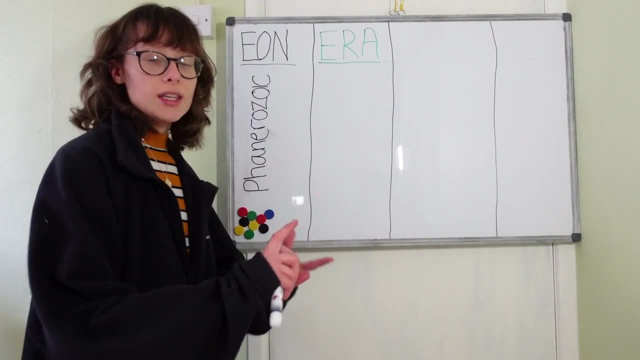 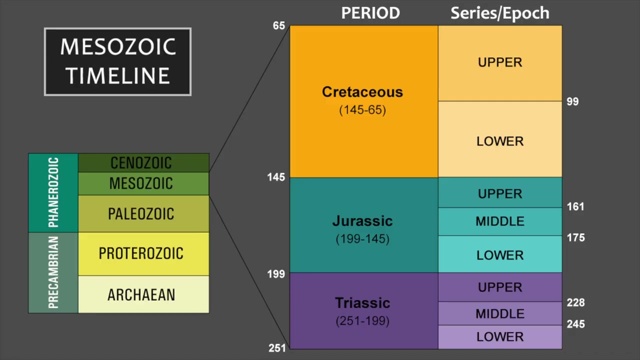 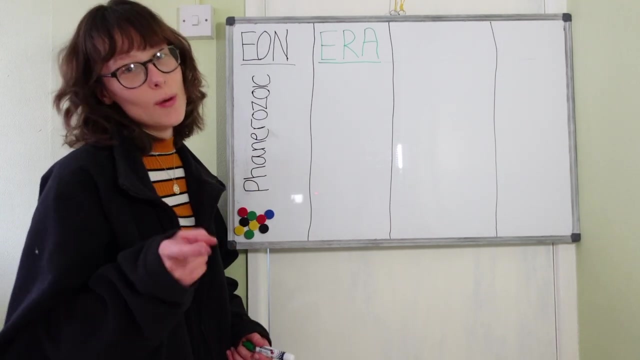 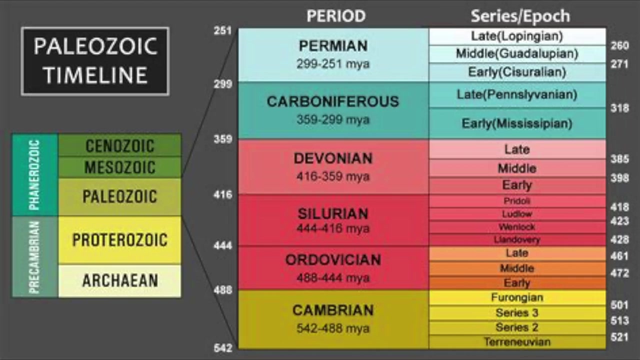 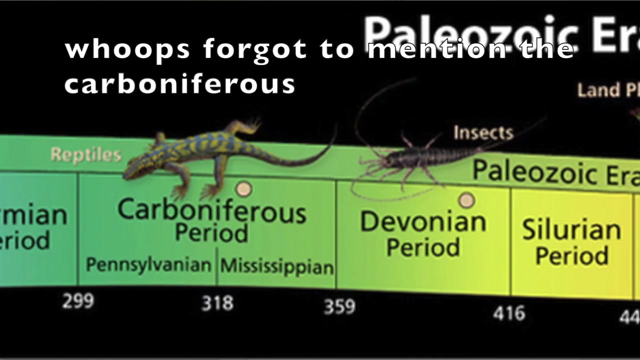 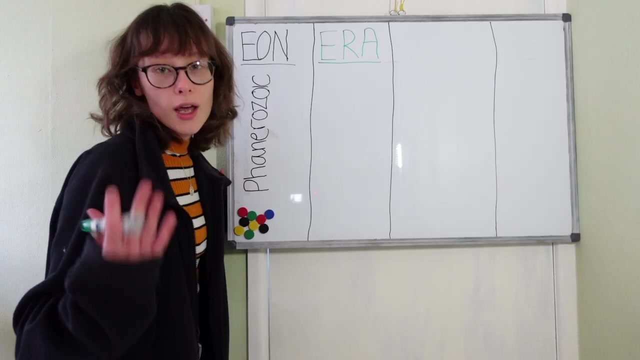 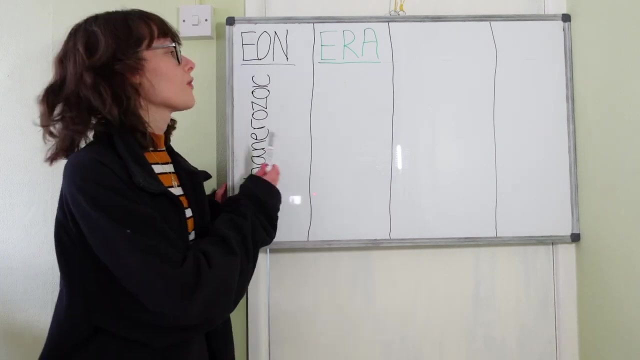 Now, eras essentially divide up time periods into groups. So, for example, we have the famous age of dinosaurs, the Triassic, Jurassic, and Cretaceous, which all together would make up one era, the Mesozoic. And that lasted from 252 million years ago to 66, when, of course, there was the KT extinction. Now, there are two other eras in the phanerozoic, which are the Paleozoic, before the dinosaurs, which includes the time periods of the Cambrian, Ordovacan, Silurian, Devonian, and Permian. And then there is the Cenozoic, which includes the Tertiary and the Quaternary periods. Now, as the age of dinosaurs are the most popular paleontological time period to study, that is the one that I'm going to be focusing on. 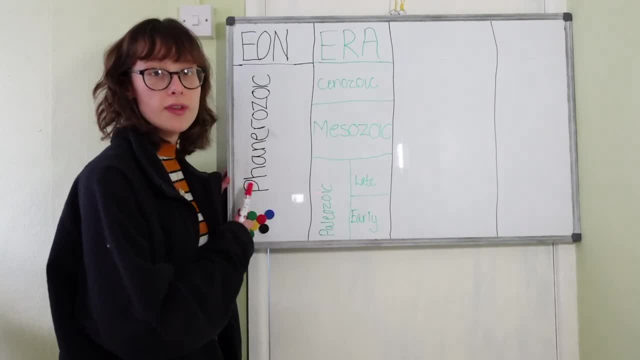 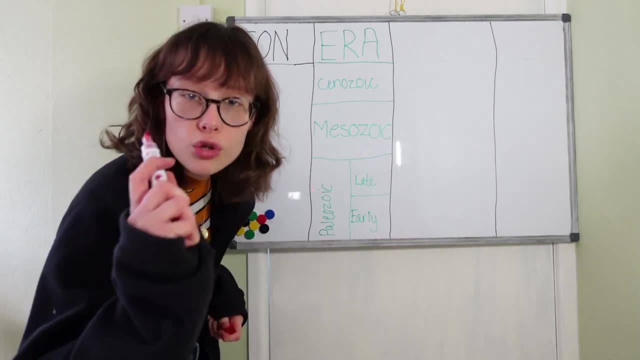 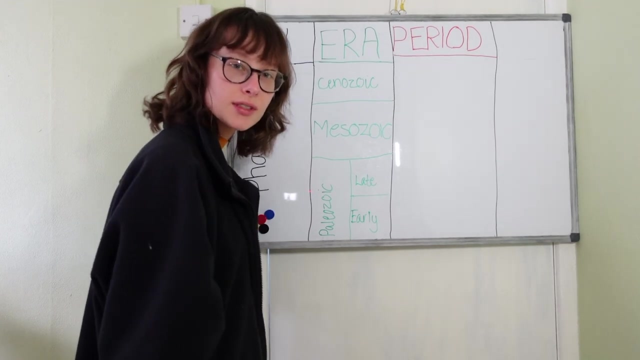 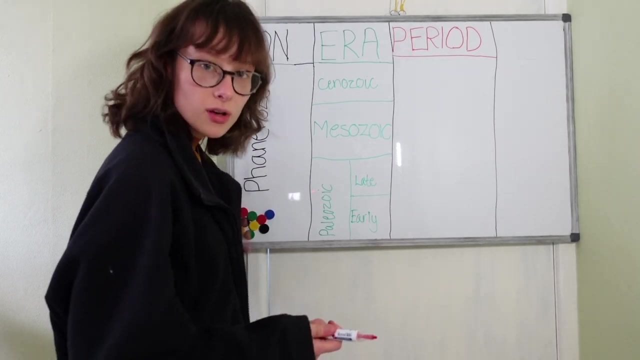 So as you can see, I've just gone and drawn out the eras of the Phanerozoic. But, as you can see, we are going to be focusing on the Mesozoic right now. So, we move on to the time periods. I just realised that I wrote period in red. So, time periods are probably the most well-known form of geological time division. And this is where we find our Triassic, 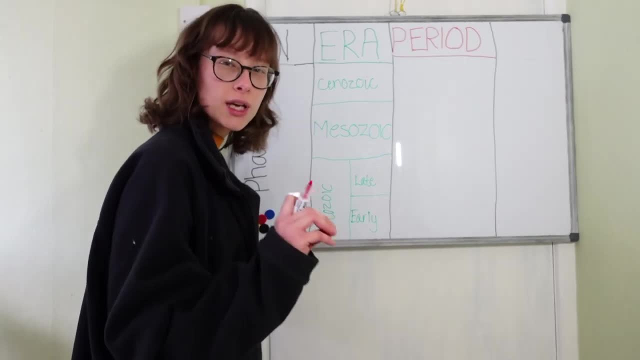 Jurassic, and Cretaceous, as well as the others. This is breaking down time into finer groups. Eras are generally more... 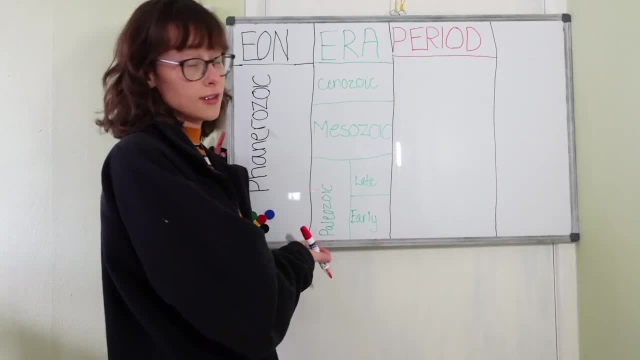 So realistic. For example, the Paleozoic, we've got the Cambrian explosion of life, 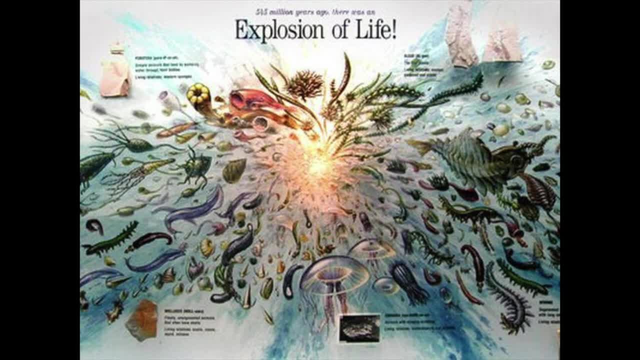 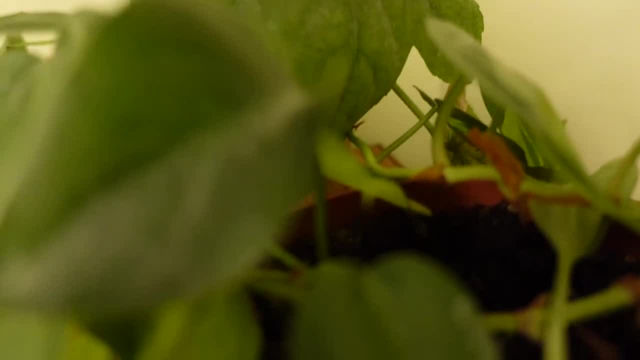 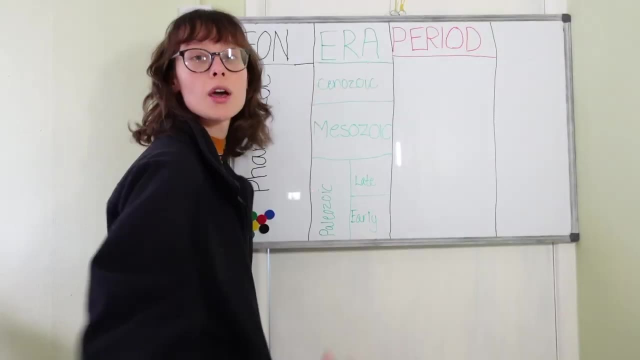 which leads on to more complex marine life forms, age of fish, plants beginning to come on land, then amphibians, insects, all of that. Mesozoic, dinosaurs. Cenozoic, mammals. 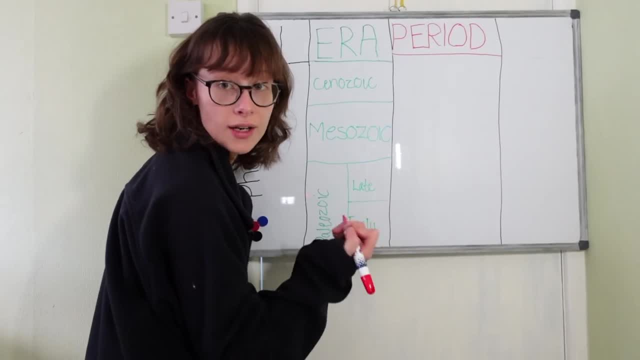 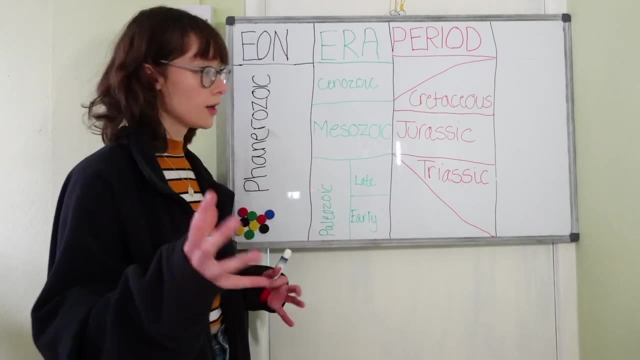 And then us, apparently. So, if I just magnify the Mesozoic for a second. In this era, we have the three time periods. So imagine we have zoomed into the Mesozoic. So, we have the Cretaceous, Jurassic, Triassic. The age of dinosaurs. Now, Triassic is when they first came about, the Cretaceous is when they died out. Good rhyme to remember. Now, each time period generally lasts for a few tens of millions of years, sometimes over a hundred, as the Cretaceous kind of almost did, lasting from, for example, 145 million years ago to 66 million years ago. Now, time periods generally split. 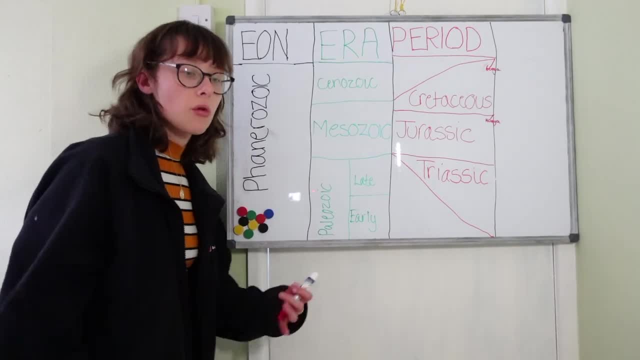 So, we have the Mesozoic, the Cretaceous, Jurassic, Triassic. The age of dinosaurs. Now, Triassic is generally split up on a basis of major changes in geological strata, as well as changes 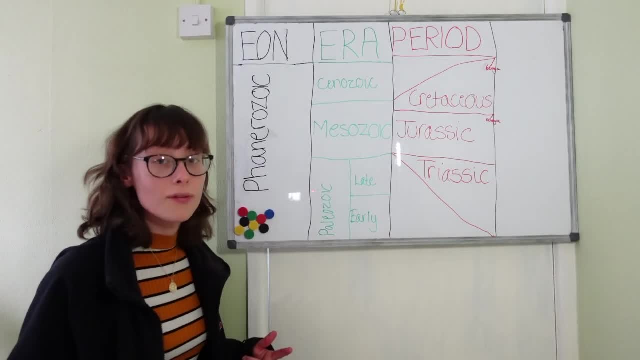 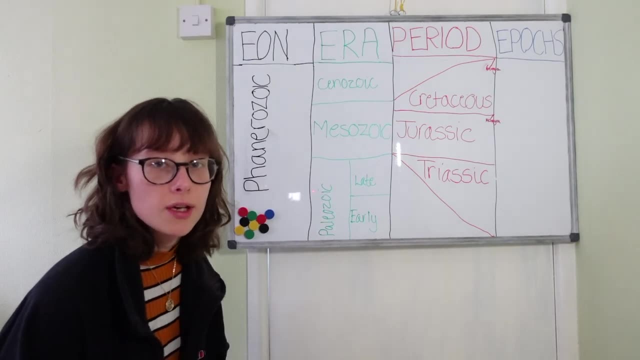 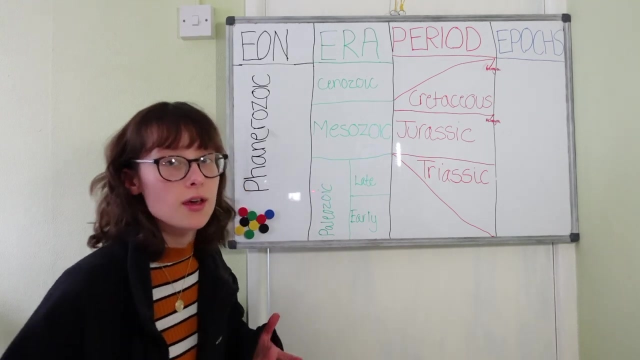 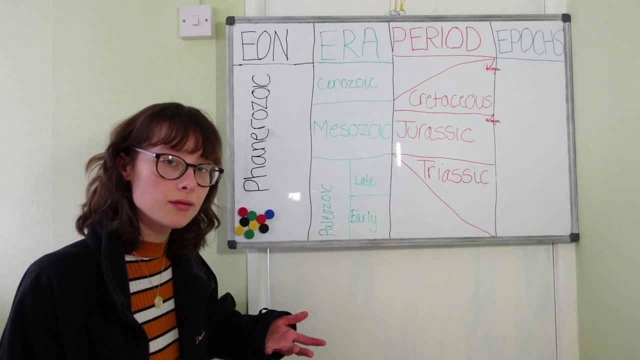 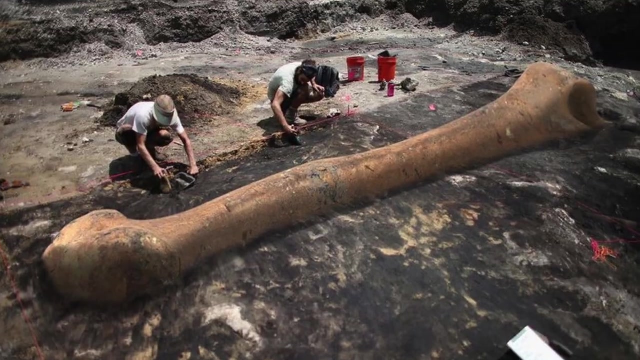 in the fossil record. So, now that we have that established, I propose we move on to epochs. So, I'm just going to sit down here for a bit because my knees are dying. So, epochs, or epochs, however you want to pronounce it, are, as you might have guessed, a further breakdown of time periods. Essentially, as you may realise, life and geology are constantly changing and geologists and paleontologists feel the need to break down time into as smaller 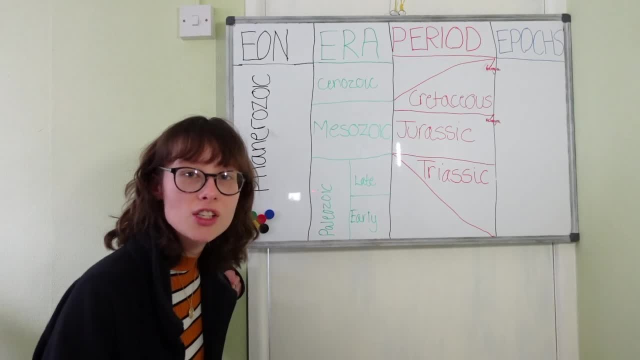 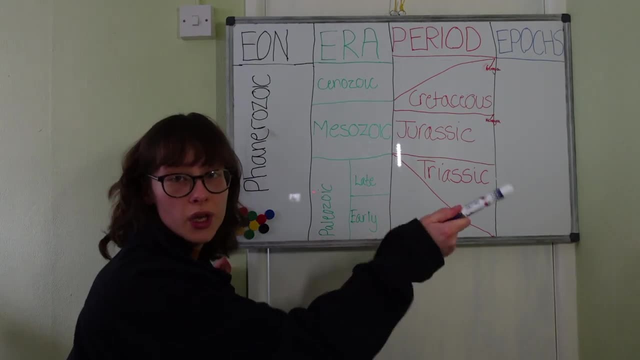 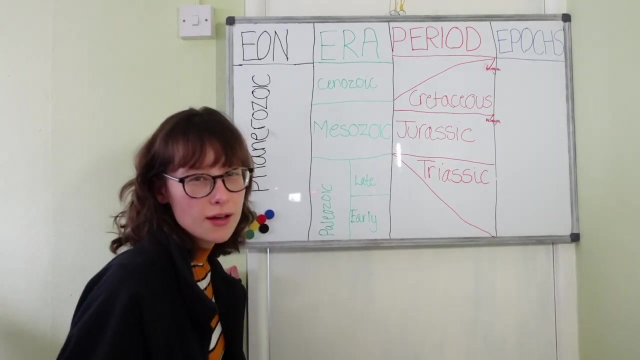 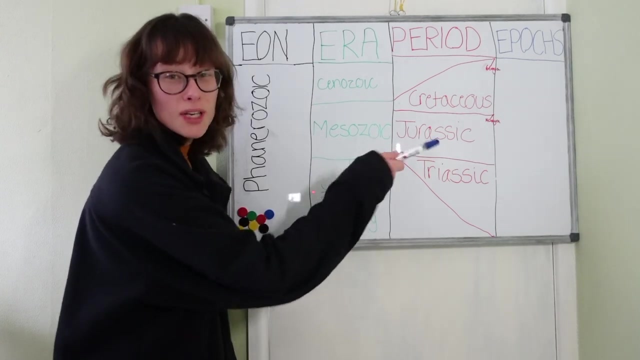 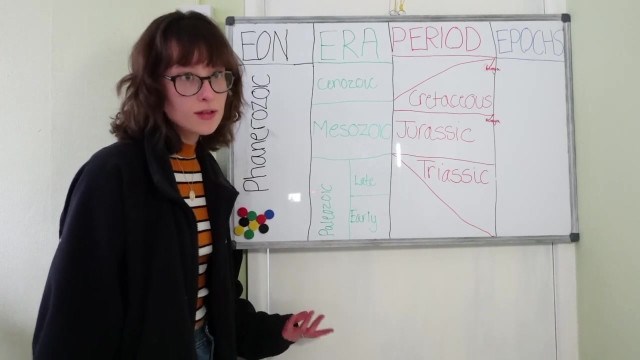 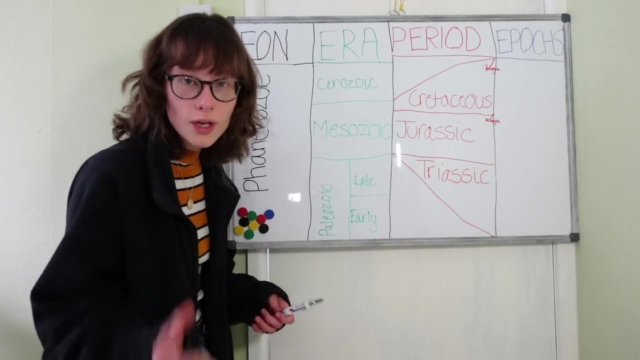 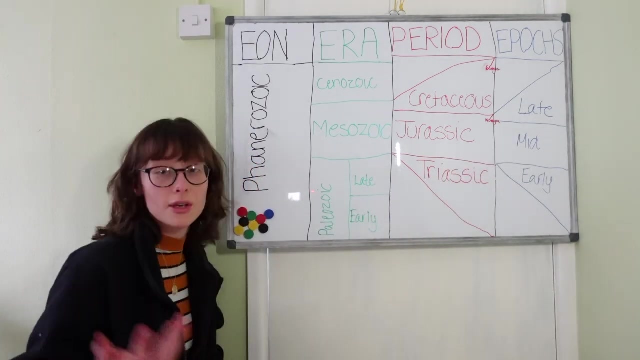 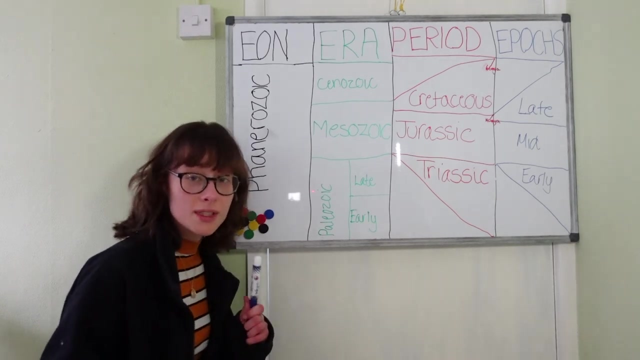 chunks as they possibly can muster. And any major change that they find, if it qualifies as not big enough for a time period, but big enough to be given a name, then it has become an epoch. Now, epochs come in various forms with various names. Some of them are simple, like in the Jurassic, when you have the early, mid and late, which is quite simple, as opposed to the tertiary, which is like Pylacene, Miocene, Oleocene, Eocene, Plezacene. I did not say those in order, but you get the gist. So, if we do a little magnifying glass once again, you can see in the Jurassic, we've got the late, mid and early. So, we've got the late, mid and early Jurassic. Some epochs, if they are that large, will again be broken down into late, mid and early themselves, which we find with some of the earlier time periods. 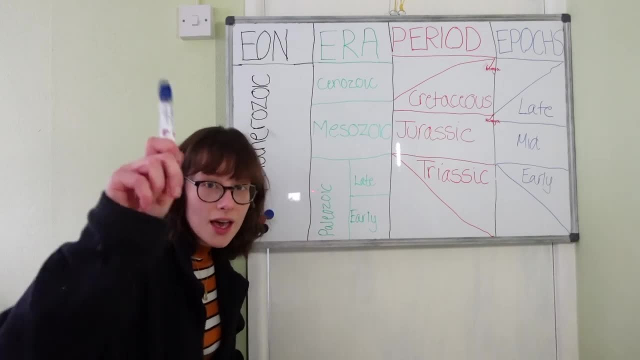 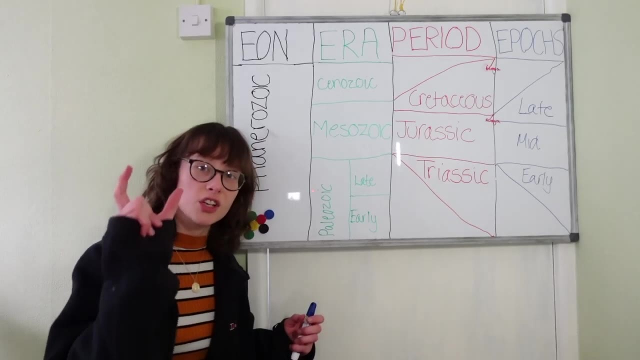 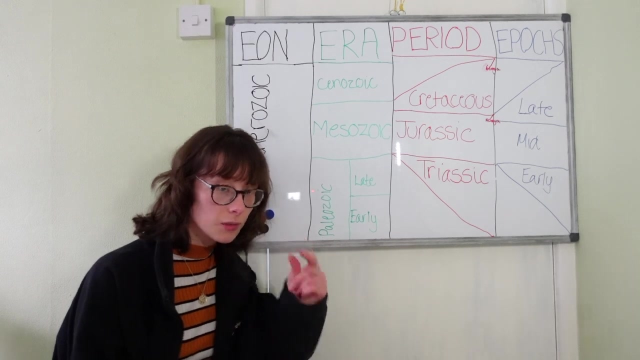 However, that is essentially that. If, again, geologists feel the need to break time down even further, then you find the geological division of ages, which I'm not going to go into because it's just like very small slices of time. I don't know.